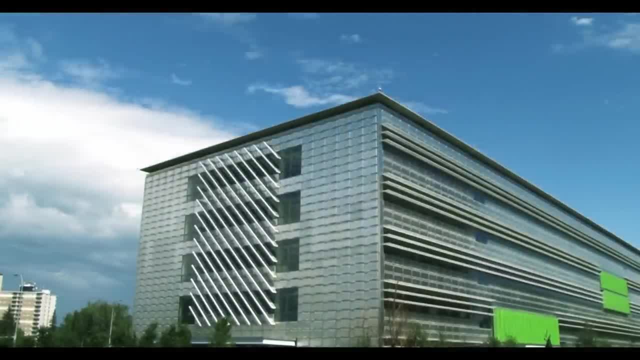 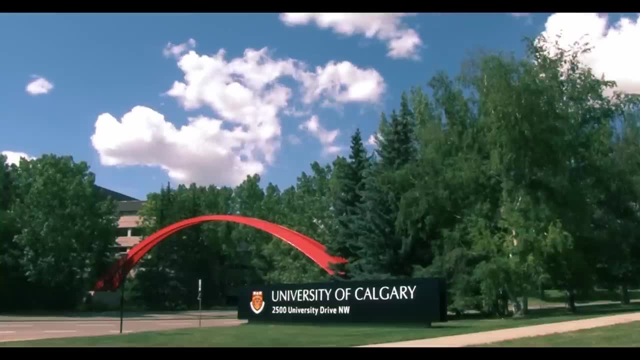 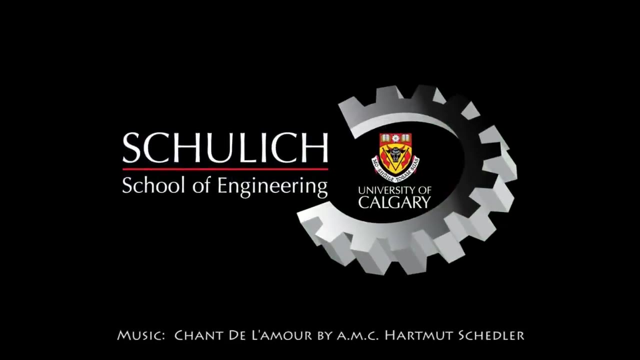 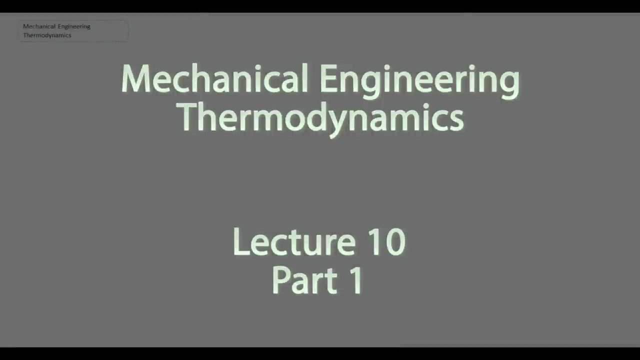 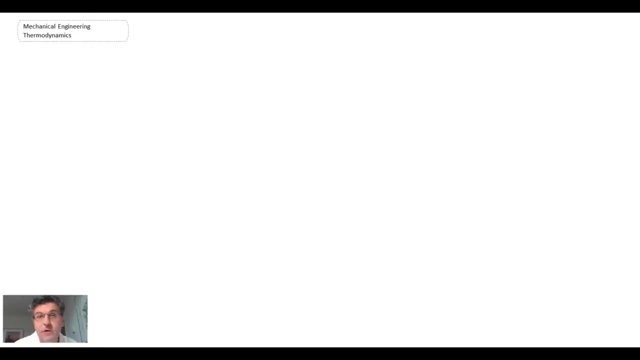 What we're now going to do is we're going to take a look at an equation that enables us to calculate the entropy balance of a system, And within this there will be a term for quantifying the amount of entropy being generated within the system, And we'll be looking at 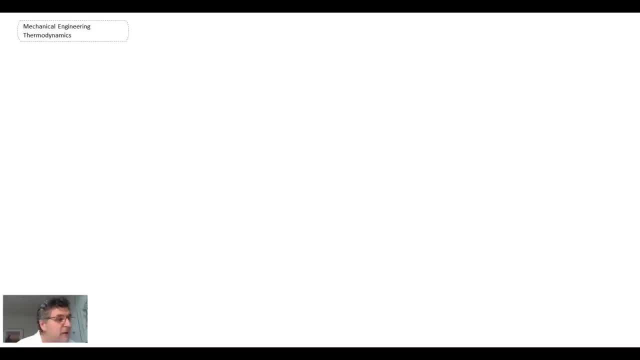 this for both a closed system as well as for an open system. Now the equation that we come up with it will enable us to compute the increase of entropy within a system, And we'll call that entropy generation. so capital S and subscript. 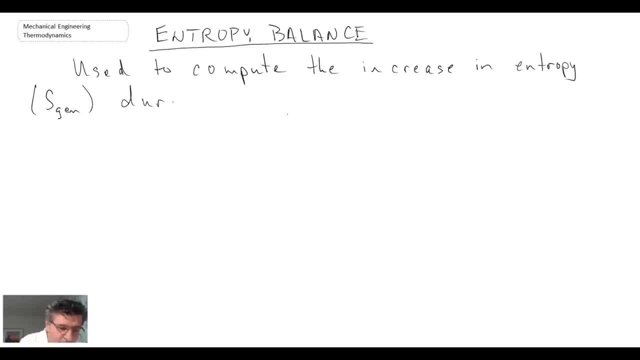 G-E-N for generation, And this would be during a system, During a process. In the previous lecture we did take a look at an example problem with the entropy generation equation, And so we've already seen a form of that, but now we'll formally present it. 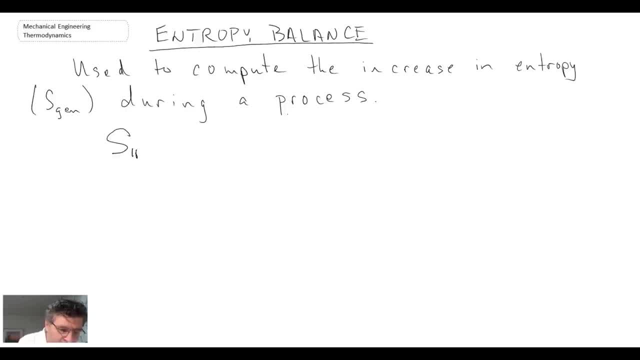 So the equation that we're working with is entropy in minus entropy out plus entropy. generation is equal to the change in entropy within the system, And the units of this equation are in kilojoules upper Kelvin. So let's take a look at the mechanisms by which entropy can be coming into or leaving our system. 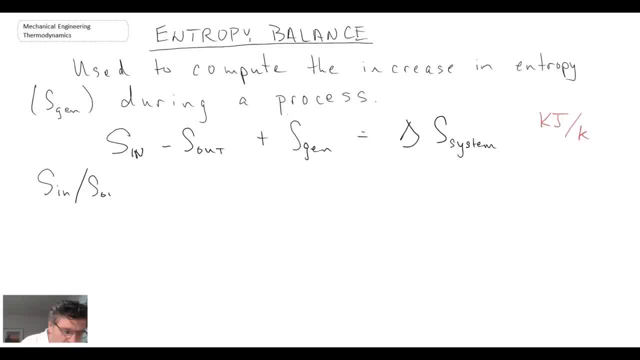 The main mechanism by which entropy will. there two main mechanisms. one is heat transfer and the other is mass transfer. And in 3D the mainvideo box runs careんと the head位待ってTYV is only a series of liquid fees or three values. it needs to become 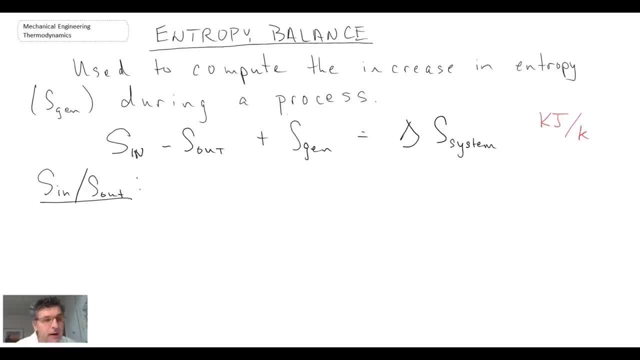 This is a second gap. This gas count needs to stay the same. Now, if the program would work- but there is, thisフ would be working, So instead we would simply have to use: Or, as you can see, for more than two attributes. 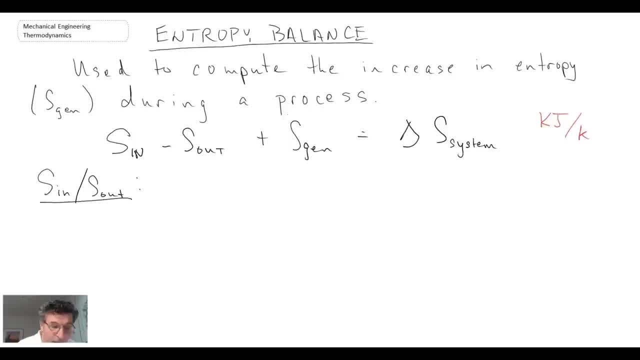 mass transfer coming into or leaving our system. So to begin with heat transfer, we write S and then small heat, Quantifying it. it is the heat transfer divided by the temperature at which that heat transfer is taking place, And so the units of that term are kilojoules. 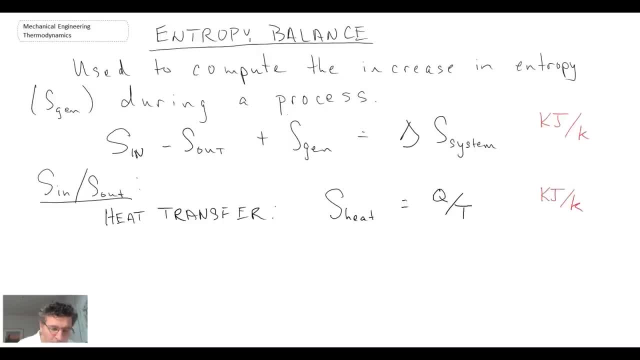 per Kelvin Work. work does not contribute to any kind of entropy generation And consequently what we can write is: entropy from work is equal to zero. And finally, mass flow. when we have mass crossing our system boundary, the mass itself can bring in entropy and it. 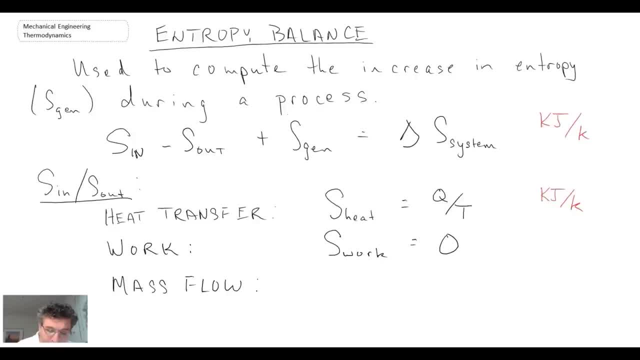 can leave with entropy And consequently we quantify that by S. mass equals to the mass times the entropy per unit mass. So the units of that particular term that we looked at there would be kilograms for the mass multiplied by kilojoules per kilogram Kelvin, which is our standard units. 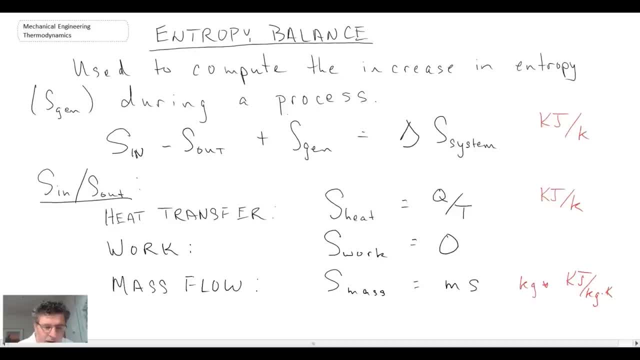 for entropy. So the form of heat transfer coming in that, remember, entropy is a quantification of the random motions, molecular motions, within our system And heat transfer is a mechanism, as we saw when we looked at conduction, whereby energy is transferring into the system. 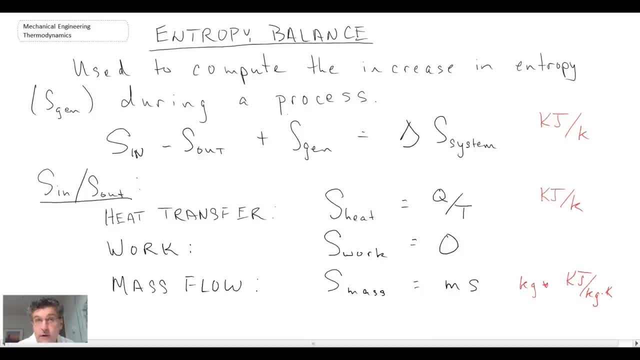 in a disorganized state. Work transfer is not disorganized, Work itself is is organized and therefore when it crosses our boundary it does not contribute to the entropy generation Mass coming in has a thermal energy, It has random motions of the molecules, It has the 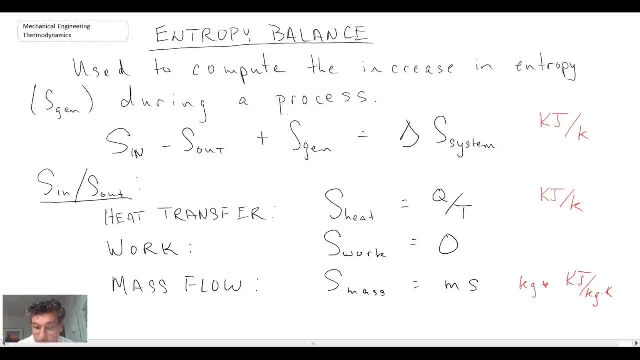 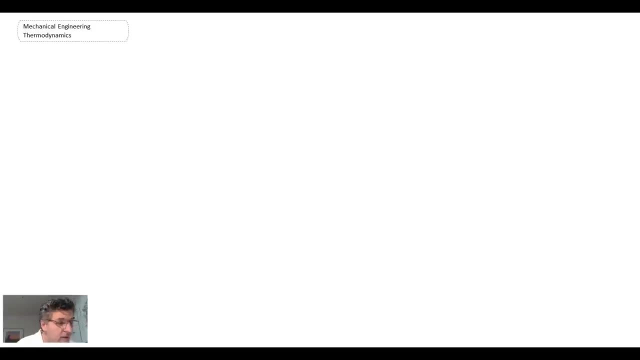 That is where it brings entropy into our system, and when mass leaves, it does the same thing: It takes it away. So that is the equation. What we're going to do now is take a look at the equation for entropy generation, both for a closed system as well as for an open system. 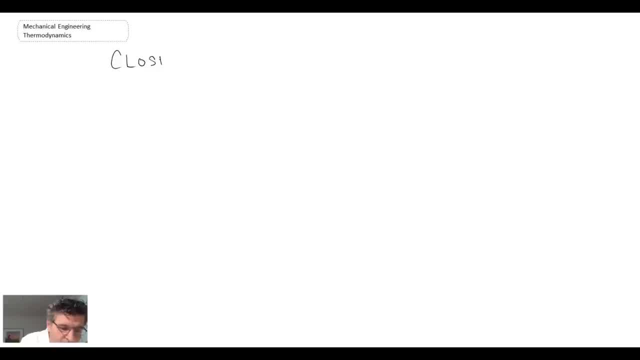 So let's look at a closed system, And this is also referred to as being a fixed mass system. So the equation for this will be the sum of the heat transfer that is taking place across our boundary plus any kind of generation, and then that is equal to the change of the system. 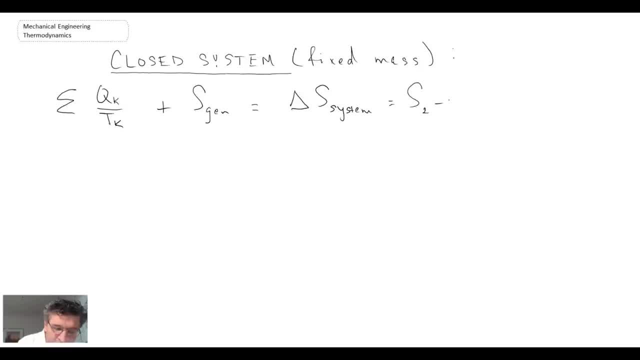 So that would be quantified by entropy. That would be entropy at state 2 minus entropy at state 1. if we were going through a process. The units of this are kilojoules per Kelvin And looking at an open system. so the control volume approach where you would have mass crossing the boundary, 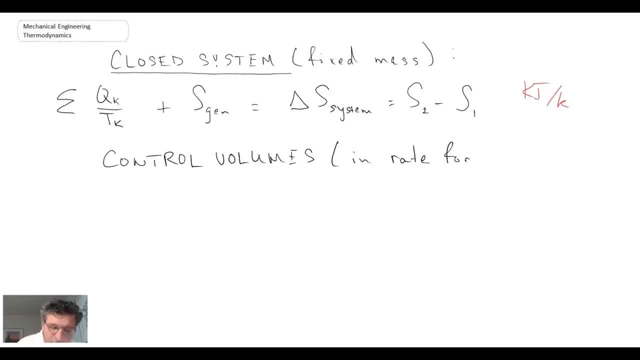 And I'm going to- I'm going to express this in rate form, and so that means that we will have mass flow rates and heat transfer rates, so that will be in kilojoules per second and mass flow rates are kilograms per second. 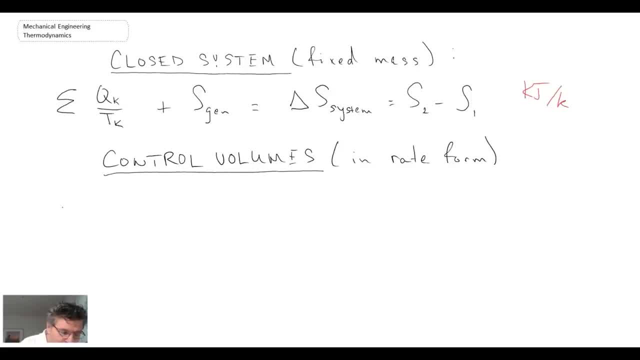 But the form of the entropy generation equation or the entropy balance. I should say, and be careful with these expressions, because the temperature In the first term with heat transfer needs to be in Kelvin. So it has to be in Kelvin, not in degrees Celsius. 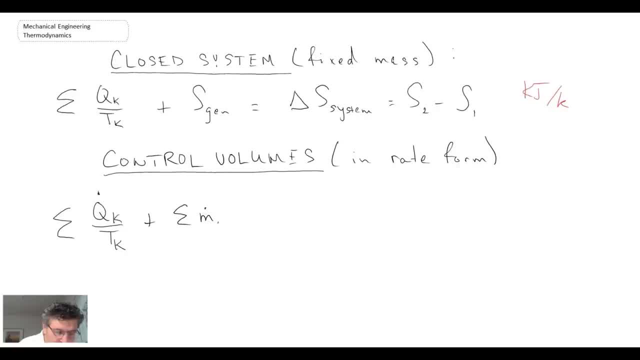 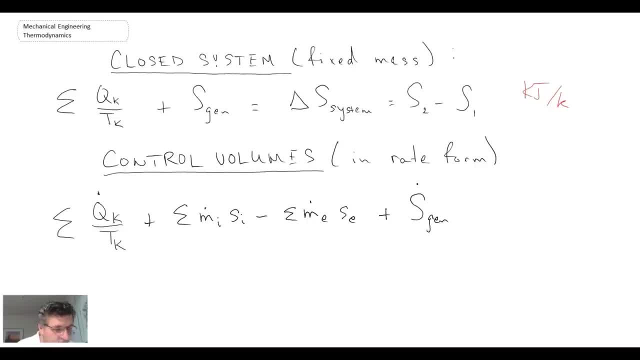 Plus generation Within our control volume, and then that would be equal to the change in entropy for the control volume, And the units of this, given it's in rate form, will be kilowatts per Kelvin. So those are two equations that we will be using to determine the entropy balance. 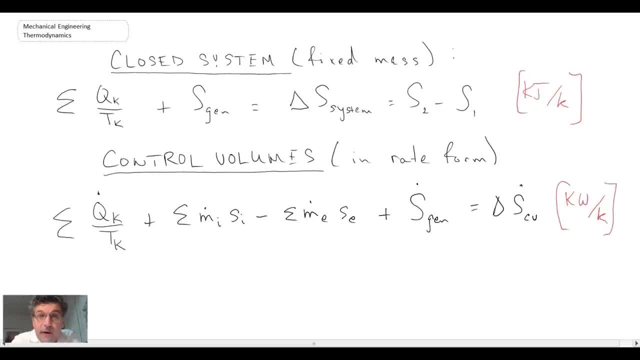 Quite often, we use it to determine entropy generation within a particular system, And this is something that we may be studying. Thank you, Thank you.